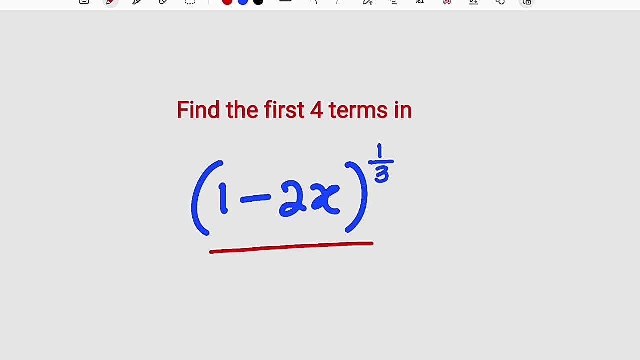 four terms in the expansion of 1 minus 2x to the power of 1 divided by 3.. We need the formula first. So whenever you have 1 plus, let me say a raised to the power of n, this is equal to 1 plus n, a plus. 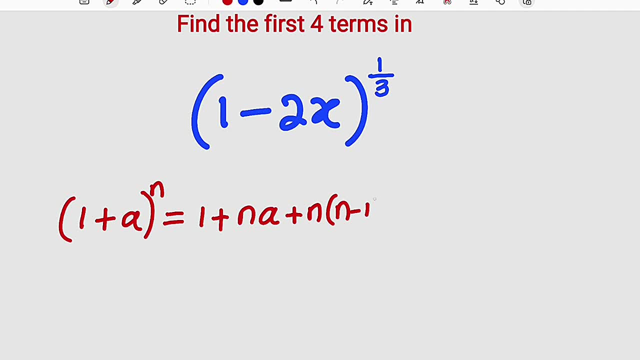 n multiplied by n minus 1, multiplied by a squared divided by 2 factorial, plus n multiplied by n minus 1.. 1 multiplied by n minus 2 multiplied by a cubed divided by 3 factorial. This is how you're going to continue adding these terms. Next will be: what Add to n minus 3 multiplied by a, to the power of. 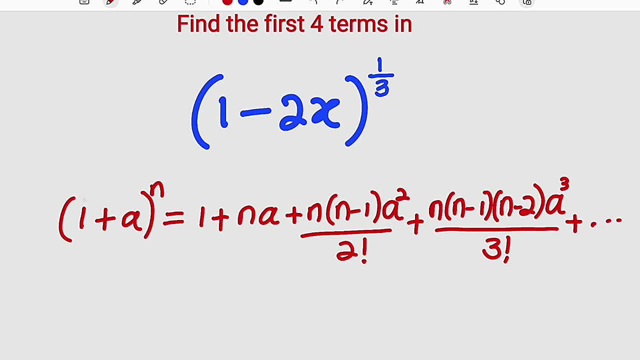 4, then divide by 4 factorial. One thing you must ensure is that the first term here is 1.. If it is not, 1, you have to convert it to 1.. All right, let us use this formula to expand this. 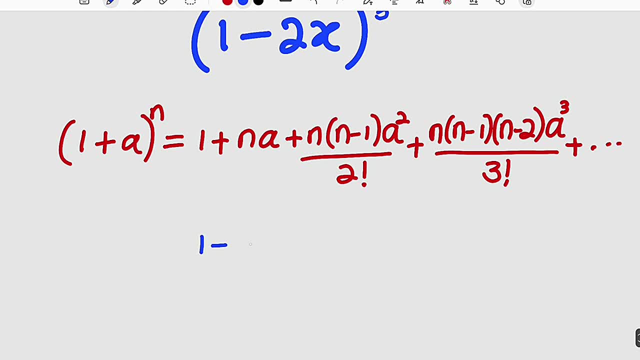 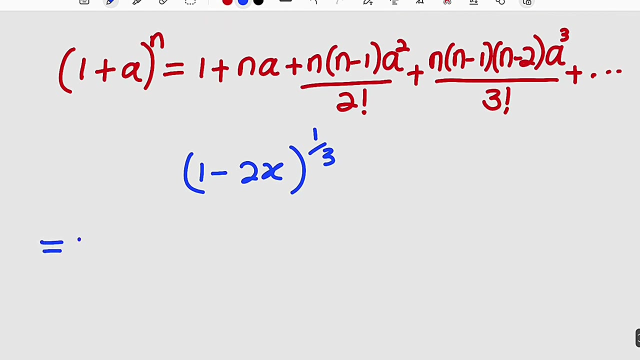 into four terms, So 1 minus 2x to the power of 1 divided by 3.. If you observe negative, 2x here will be our a and 1 divided by 3 will be our n. So this is equal to 1 plus n, which is 1 divided by 3.. Then multiplied, 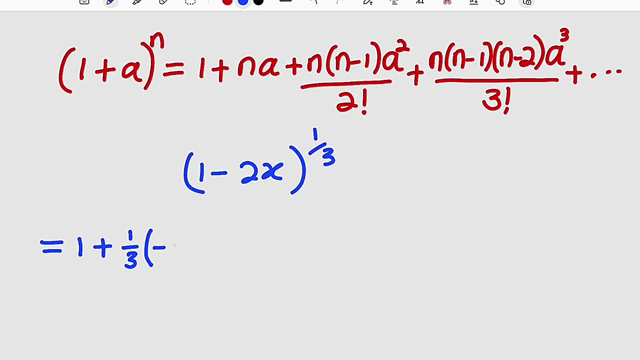 by a, which is what? Negative 2x, Negative 2x. We have first and second terms, Right Plus n, which is 1 divided by 3 multiplied by n, which is the same thing as 1 divided by 3 minus. 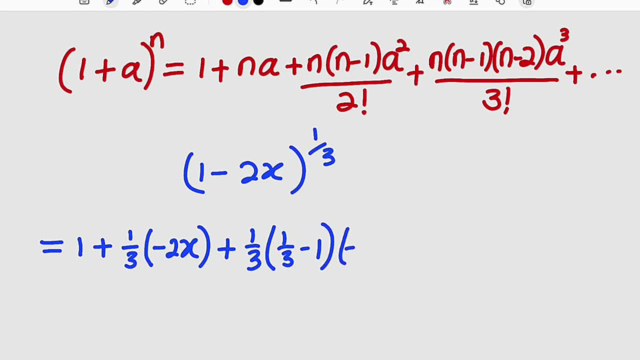 1 multiplied by a squared That is negative, 2x all squared divided by 2, factorial Plus n, which is 1 divided by 3 multiplied by 1, divided by 3 minus 1, multiplied by 1 divided by 3 minus 1 multiplied. 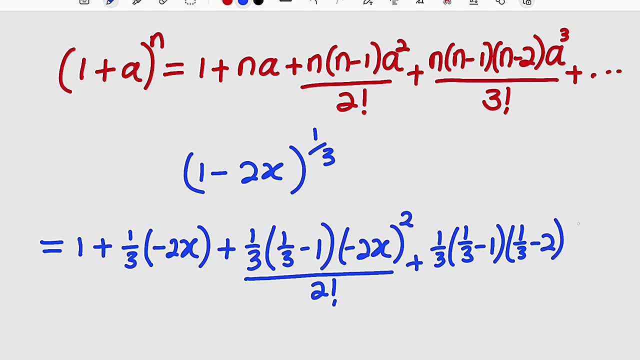 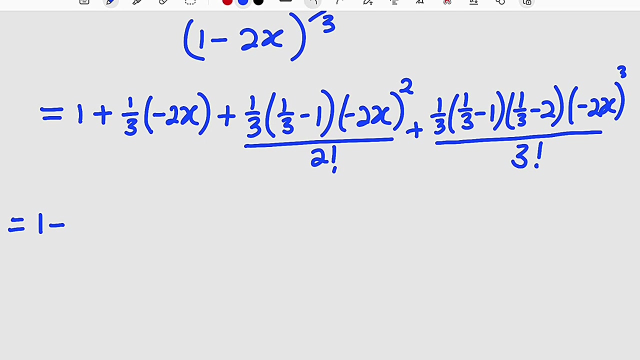 by 1 divided by 3 minus 2, multiplied by a cubed, which is negative 2x to the power of 3 divided by 3 factorial. i think these are the first four times we have. let us simplify them. this is equal to 1 plus. okay, this will give us minus because we are multiplying together. 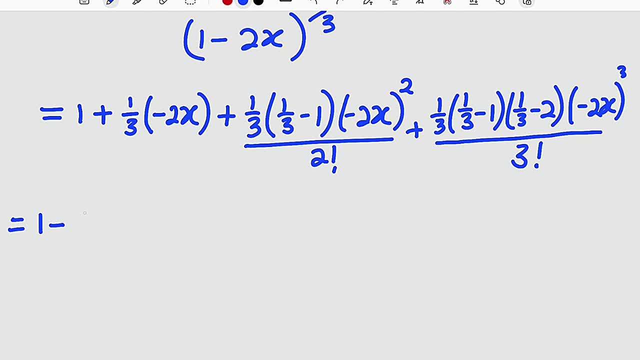 1 over 3 times negative 2x will give us negative 2x divided by 3. then we move to the other terms. 1 over 3 minus 1 is the same thing as negative 2 divided by 3. we have 1 over 3 outside waiting. 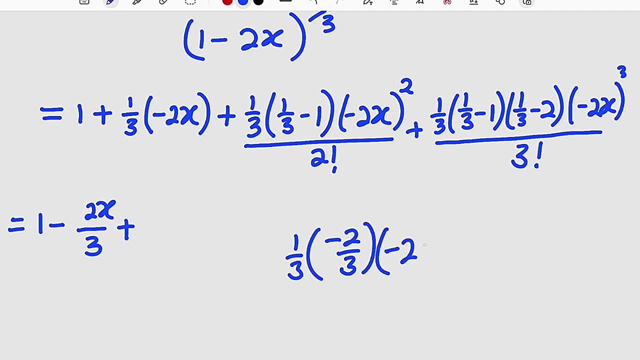 to multiply. then we have another negative 2x squared, which is going to give us what 4x squared. so let me write 4x squared. i want to simplify everything. you. then, if you multiply all this together, i have negative 2 times. 4 is negative 8. 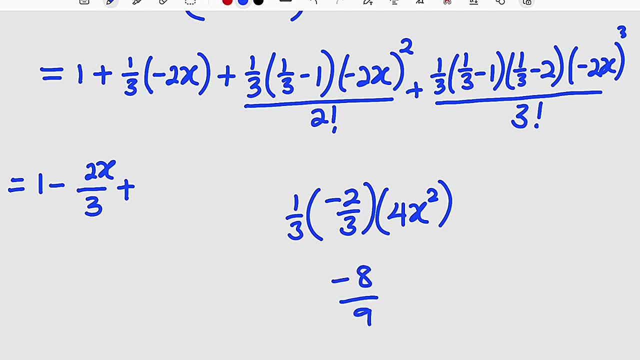 this is negative 8 divided by 9. right, so we have negative 8 divided by 9. don't forget the x squared here. but we have to divide by 2 factorial, and 2 factorial is the same thing as what 2, so it's like we are multiplying by 2 here. let us take the last term. 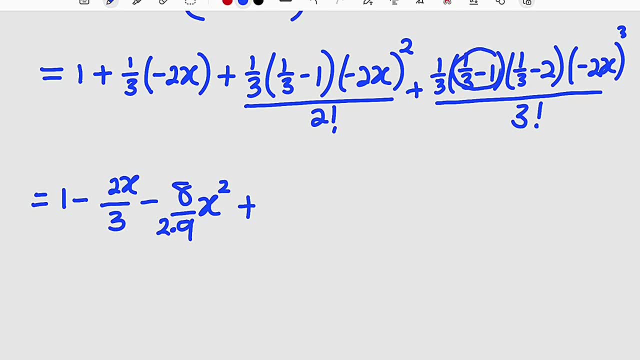 plus. already we have seen that this is negative 2 divided by 3. so we have one divide by 3 multiplied by negative 2 divided by 3. now what is 1 divided by 3 minus 2? is negative 5 divided by 3, negative 5 divided by 3. then we have another 1 negative 2. 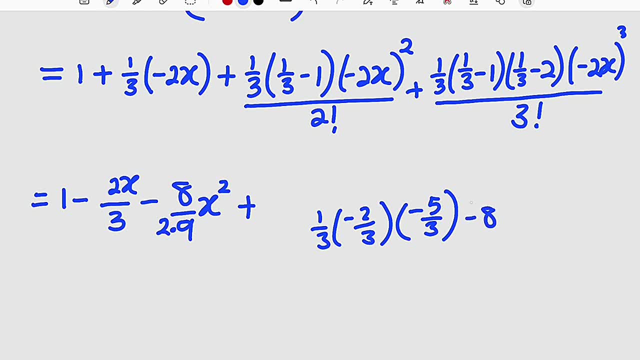 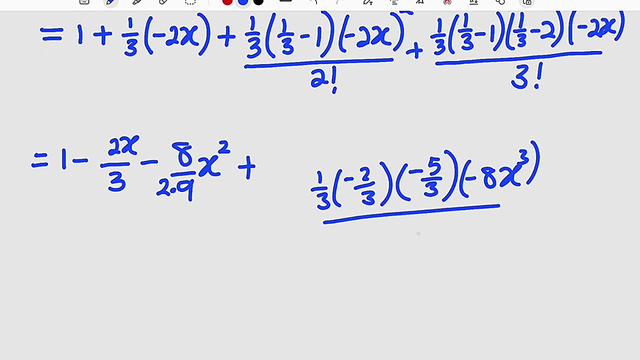 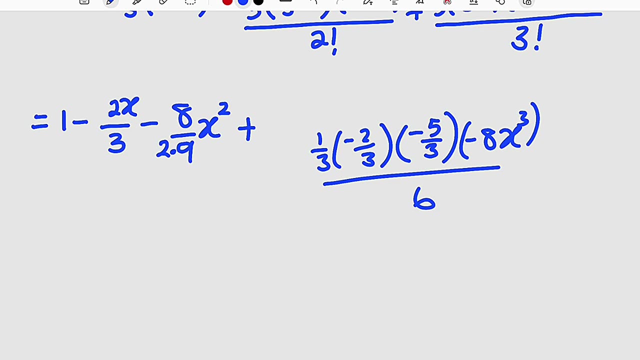 x to the third power is negative 8, x to the third power. so let's multiply all this together. don't forget to divide by 3 factorial, which is 6. let's multiply the top negative. 2 times negative, 5 will give us positive 10, and 10 times negative, 8 is negative 80. so we have negative 80 divided. 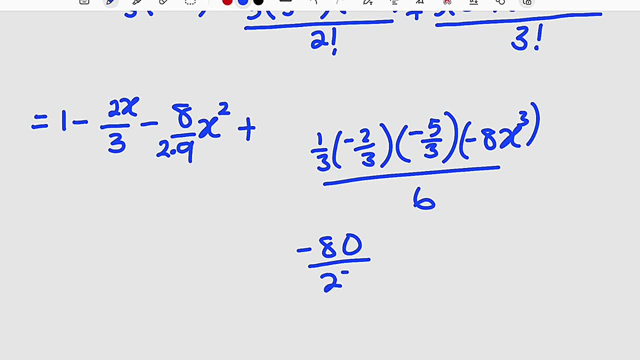 by 3 times. 3 times 3 is 27, but don't forget to multiply by this 6. so this is negative 80 X to the third power divided by 162. so we have negative 80 X to the third power divided by 162. let us: